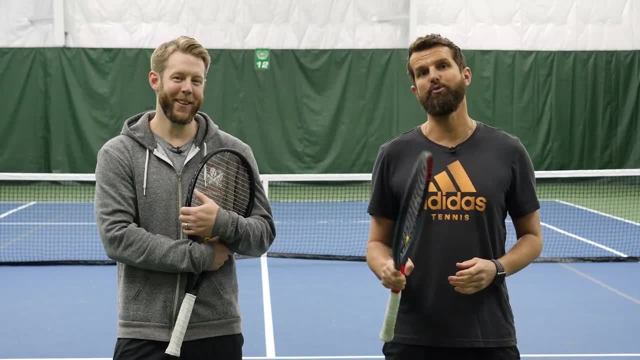 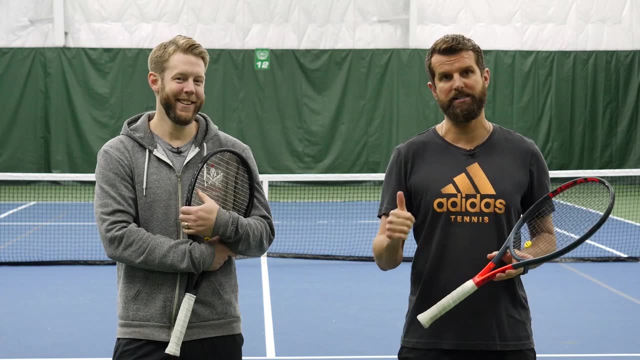 Hey y'all, how y'all doing. This is Nate from PlayYourCourtcom, here with my infinitely better looking friend, Scott, And today we're going to talk about forehand spacing. and it's a good thing, because Scott's forehand is just so much gosh darn better than mine, I think. 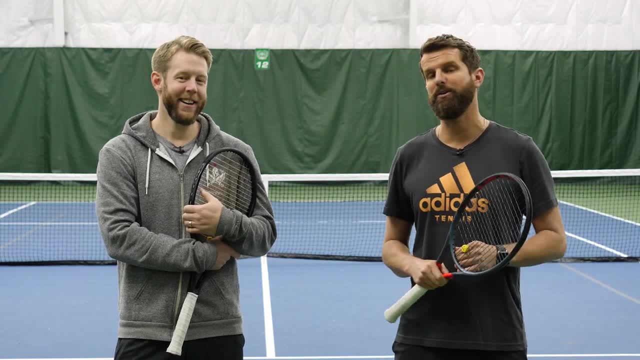 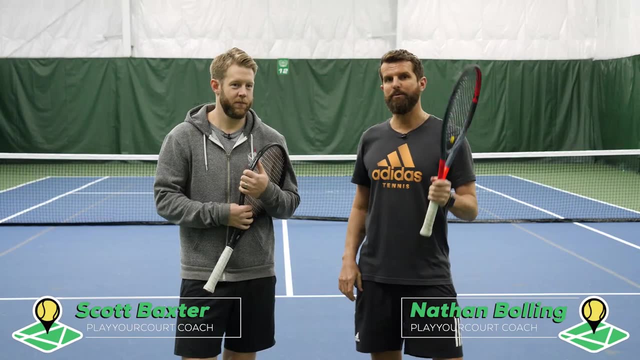 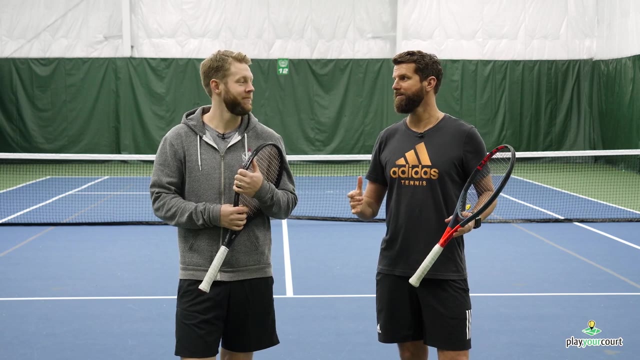 you guys are going to especially like this video because it's a lot more of Scott than it is of me. Alright, guys, so today we're talking about proper spacing on the forehand, and this is everything, because, regardless of how good, It's especially important. 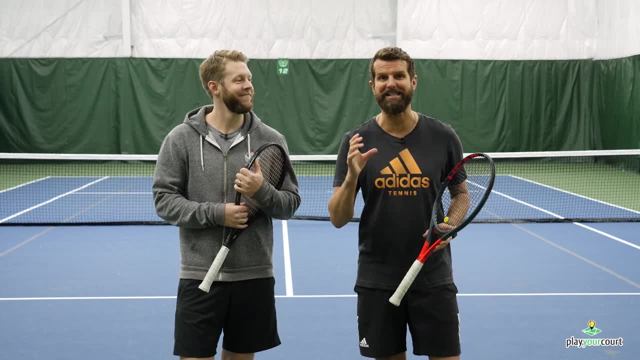 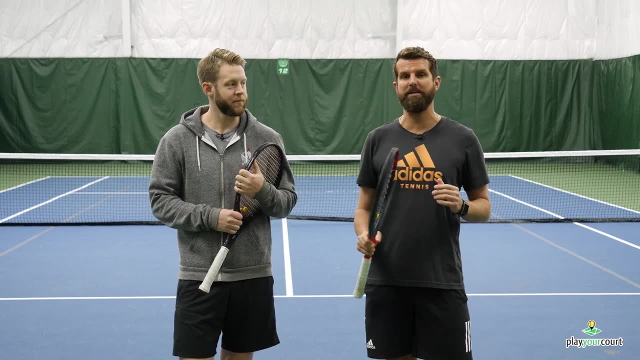 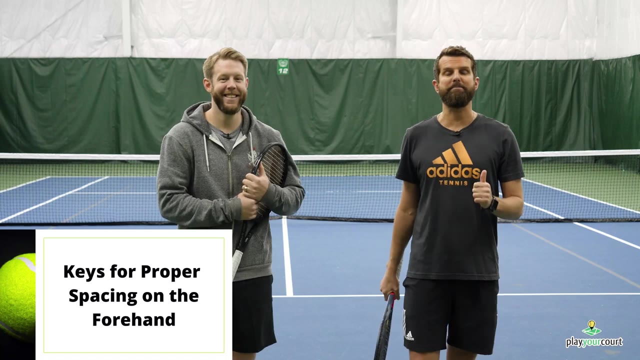 Regardless of how good your timing is, if your spacing is off it's going to cause problems, And there's a couple things, little parameters, that we can set to make sure our spacing is especially good, Especially good, Especially Alright. so number one is making sure that you get your outside leg behind the ball. 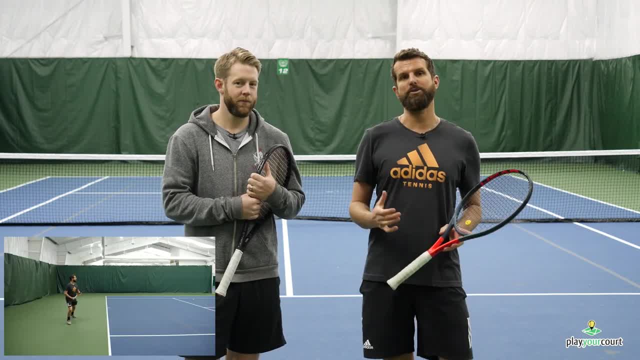 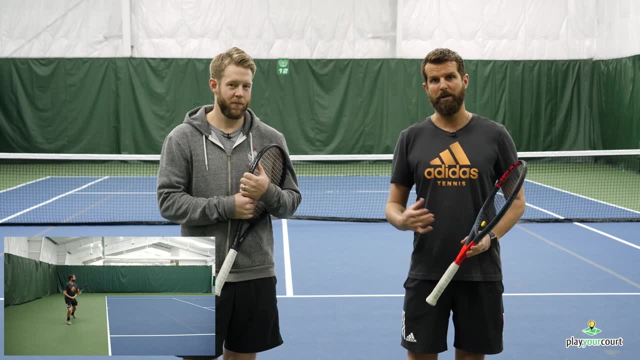 So, as you can see in the demo here, every time the ball is being struck, I'm working on getting my outside leg- the leg that I'm loading- I'm coiling on behind the ball. Alright, if, for any reason, that leg's not behind the ball, I'm going to be off balance. 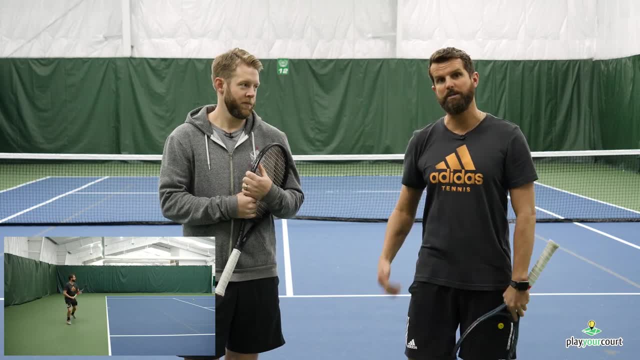 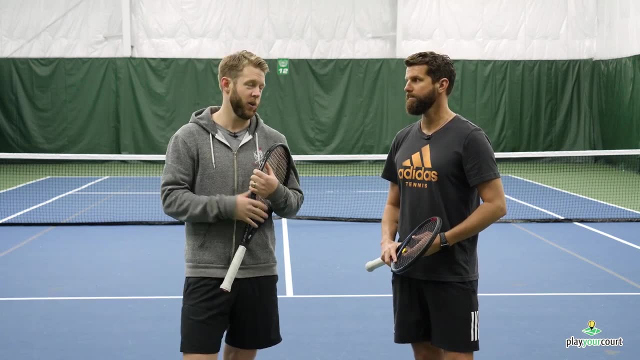 I'm not going to be able to corkscrew and then really work through that on coil to deliver the power back. This really is the foundation of a balanced forehand too, so don't discredit this. This is more important than I think a lot of you give it credit. 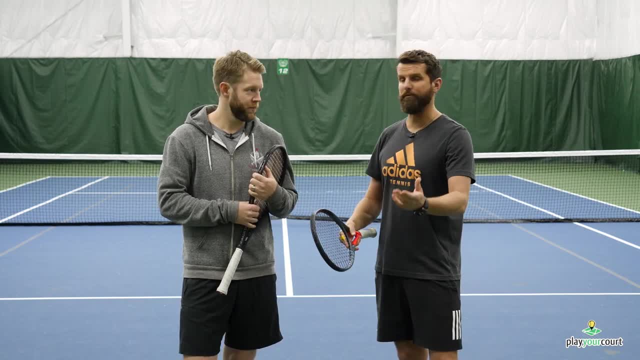 It's huge. Alright, and I know you may be thinking: well, what about getting on your front foot? Absolutely, If the ball allows me, If Scott's incoming ball, my opponent's incoming ball, is short or very short, I'm going to give. 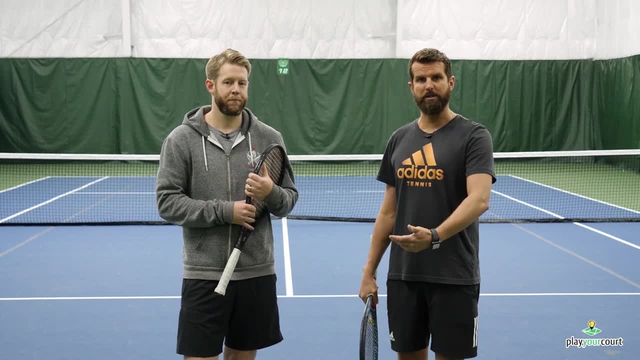 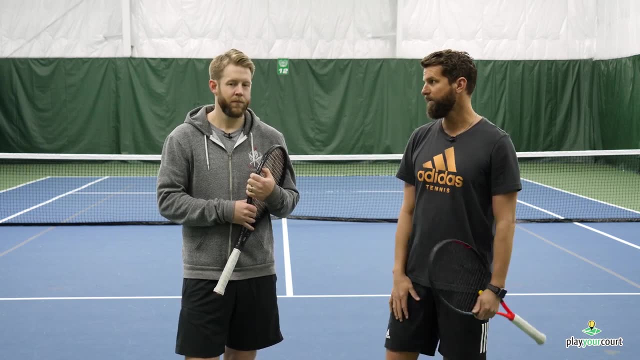 it credit If it's weaker. absolutely, I would work to step in and be a little bit more aggressive off this front foot, but right now it's about absorbing power and really delivering it back. Step two is just a quick reminder for spacing right. 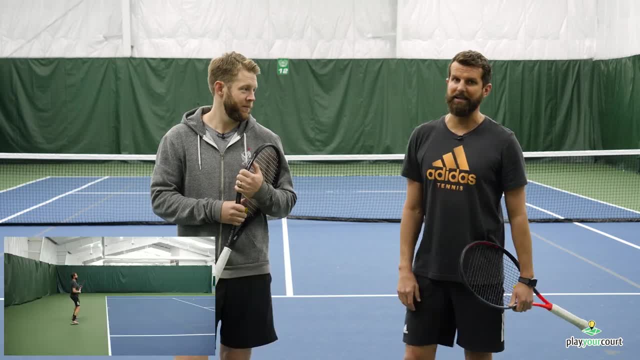 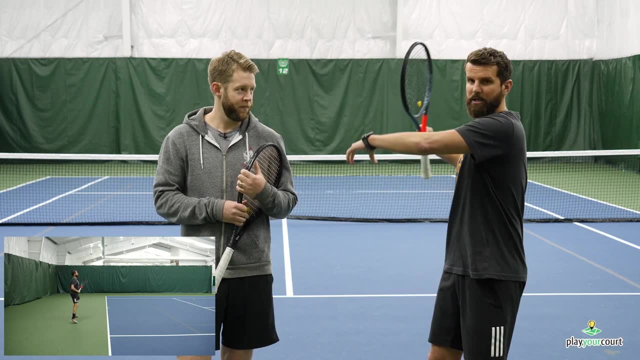 Yep, Talking about our left hand. as a right-handed player, A hundred percent That left hand. we really want it horizontal, okay. So not only we've done a bunch of videos where we've talked about getting the left arm out because it helps the unit turn, helps our shoulders get turned, but it's also about 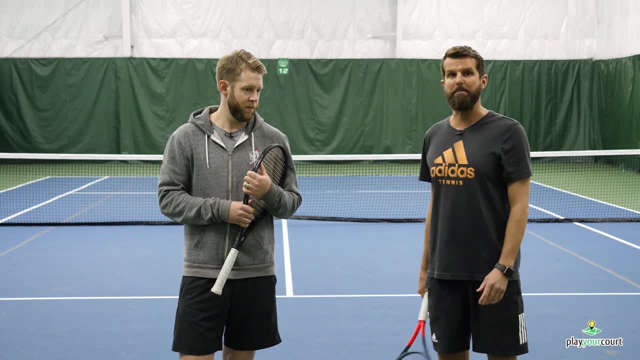 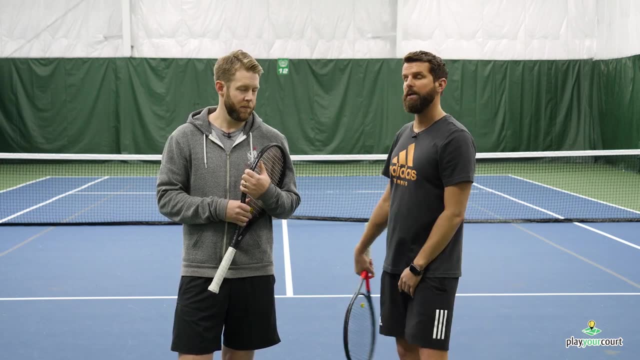 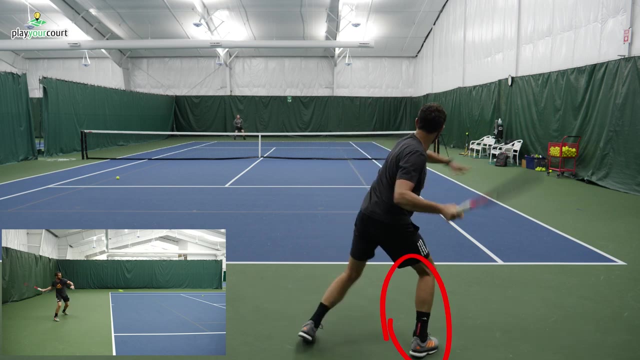 spacing okay, And we're going to show you a cool little drill to make sure that we understand exactly how this left hand and how the right foot coordinate and work together to keep the appropriate spacing All right. so here we're taking a closer look, really investigating these parameters being 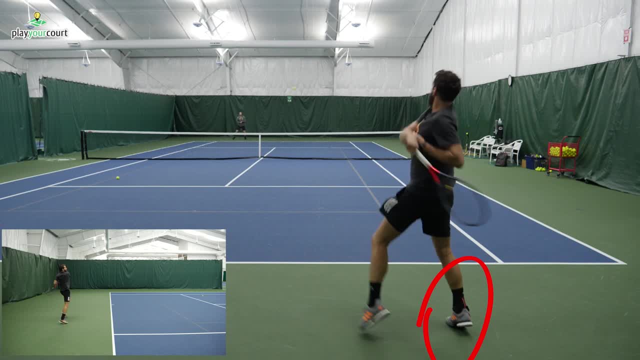 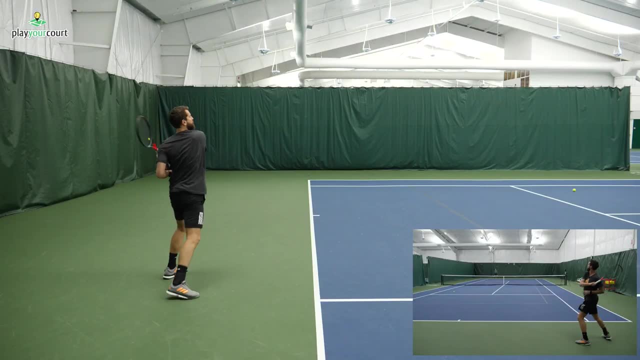 set for this proper spacing. And the first, as you can see, is the loading of the outside leg. The right leg is a right-hand player really loading it and- something important to note here- The left is parallel with the baseline. 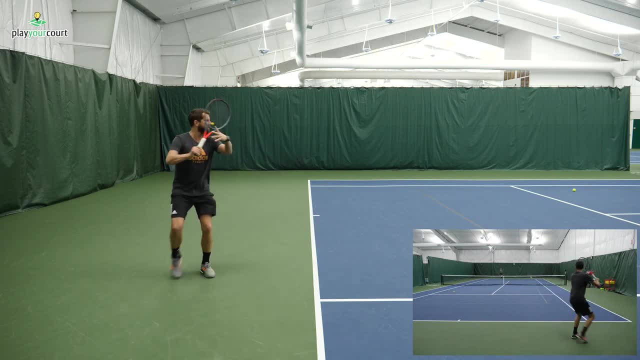 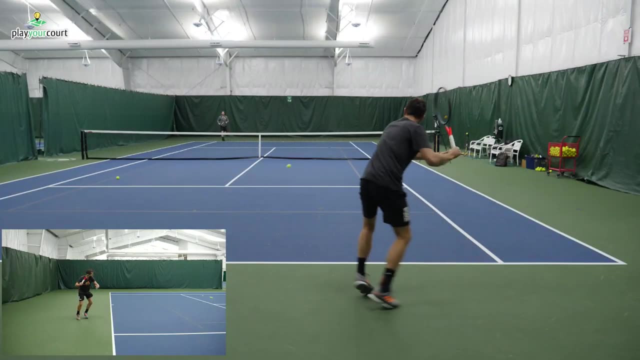 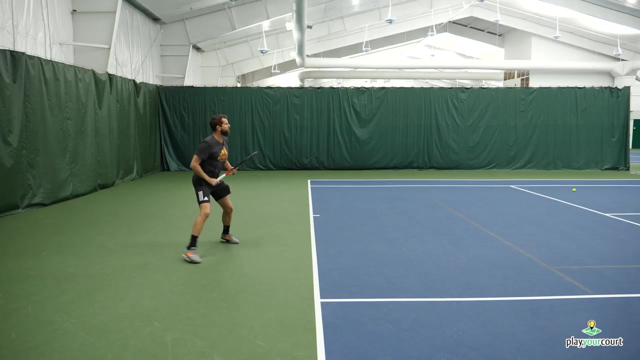 It can be offset just a little bit slightly diagonal, but it's really important that the toe faces out towards the curtain, because this is going to help keep the shoulders closed longer, so you don't over-rotate. The second thing that we're going to really look at here is the left hand. all right. 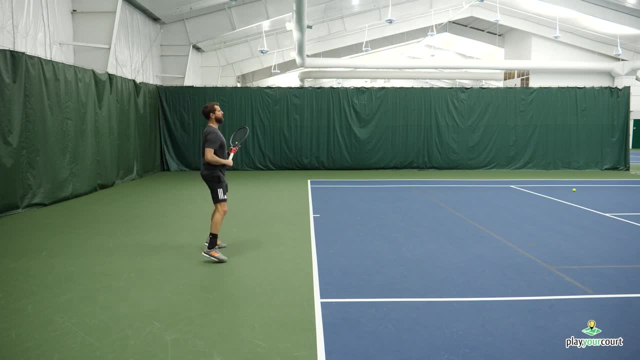 It's as if that left hand is reaching across, pushing out towards the opposing wall and this is ensuring that unit turn. Okay, It's making sure that ball stays on the outside of the body so that the racquet can get through the swing path and extension, giving us proper contact. 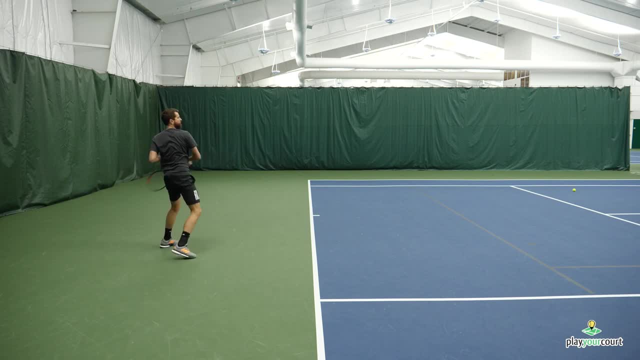 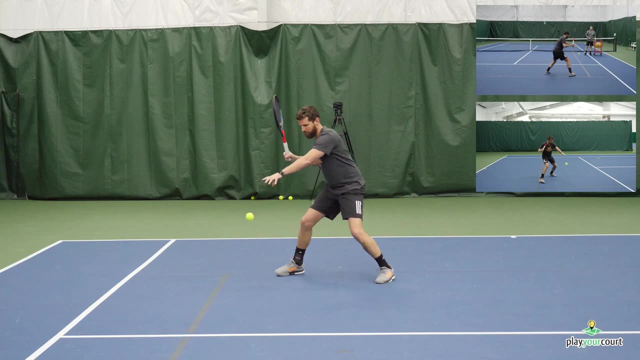 Okay, so here we got a drill that's really really good at understanding. the spacing forces us to get that non-dominant hand and loading on the outside leg With Scott using hand-fed. he can control the parameters of the drill, but it still. 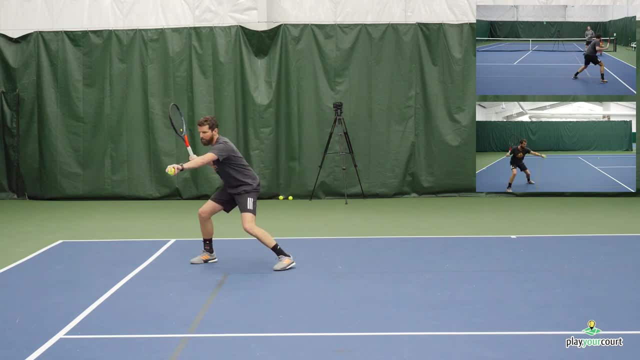 forces me to get that non-dominant hand and loading on the outside leg. I can get more of that right here and I can actually actually get the ball in defense when I do drop feed. It's really important for me to track the ball, keeping the ball on the outside staying. 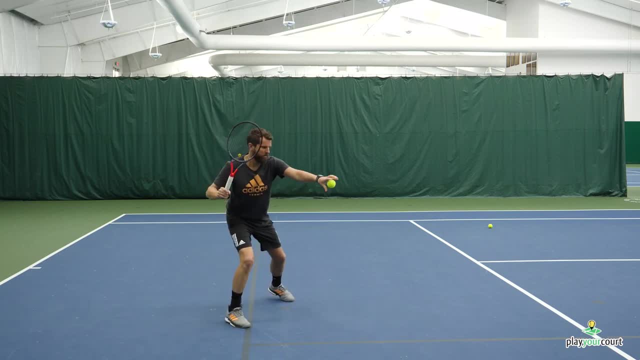 focused on where I want the contact with the drop feed And I can really start visualizing what this should look like when we go live. It's one of our favorite drills to use with our students and it's certainly something that you can get out and practice. 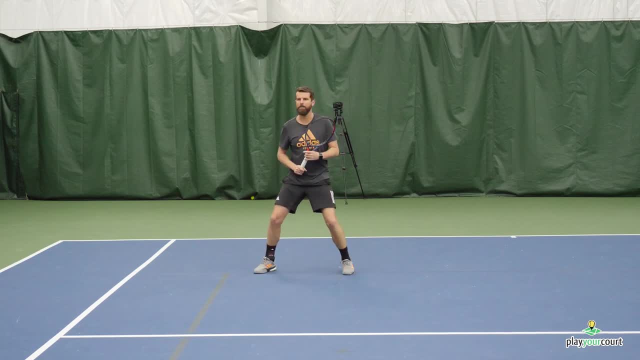 And you can do this with just a handful of balls. You don't have to necessarily have someone feeding right. If you drop the ball to the side, make sure you get that left hand out, make sure you get your leg behind it and then work through the stroke. 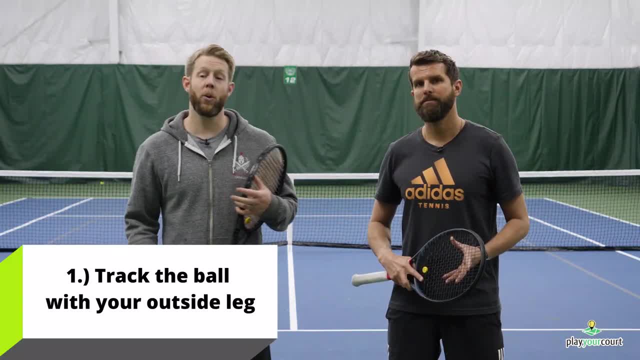 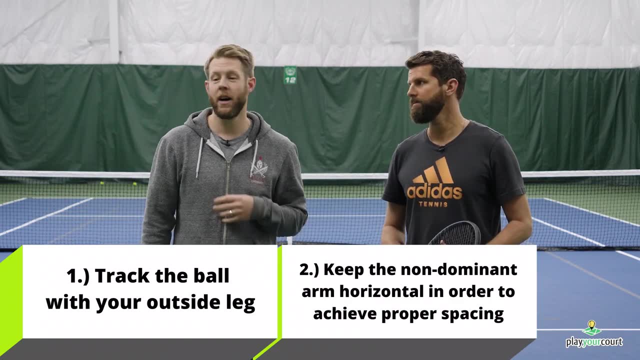 All right guys. So, in summary, make sure you're using that right foot- or left foot, if you're left-handed- to get behind the ball and get that foundation, and then using that left hand- or right hand, if you're left-handed- for spacing, to figure out exactly. 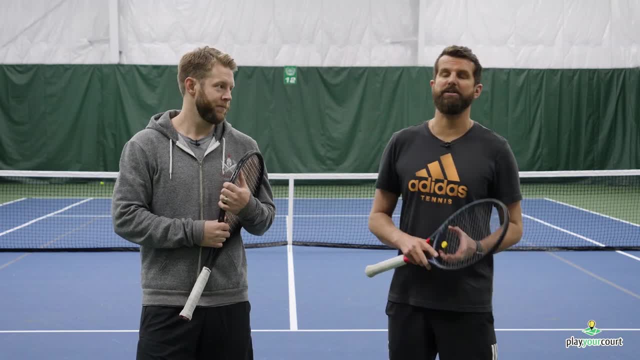 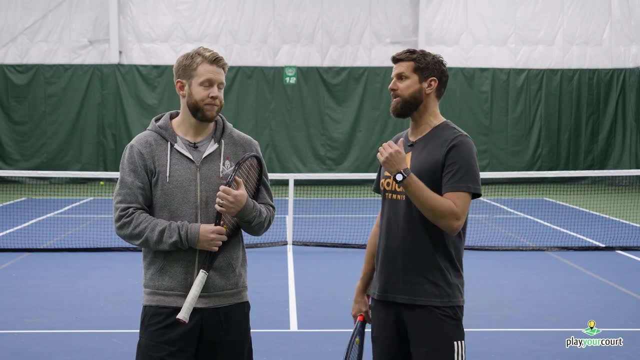 where that ball should be relative to your body And guys. this instruction is fairly general for most skill sets. It's gonna help pretty much everybody, but not all instruction is this general. Inside the community we have very specific instruction that is tailor-made just for your skill level.